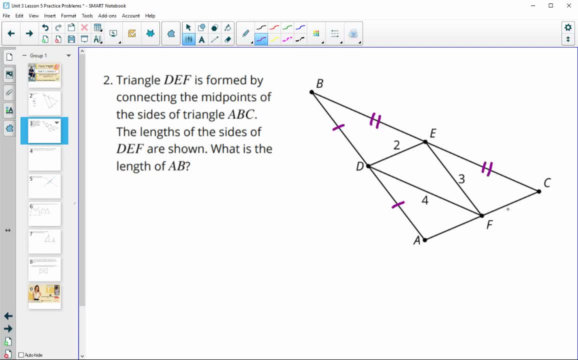 that we know that those two pieces are the same. If F is the midpoint here, then these two are the same, and what that does is gives us all these little congruent triangles, and we also know that, so we're looking for this side length. we also know that that side length is composed of: 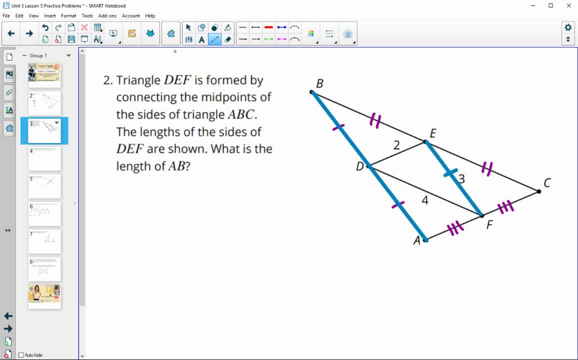 two pieces that are equal to this one, so this one is 3, and so each of these, from B to D, is 3, and D to A is 3,, and so we know that the whole length of AB is 6,, so it's kind of like it's. 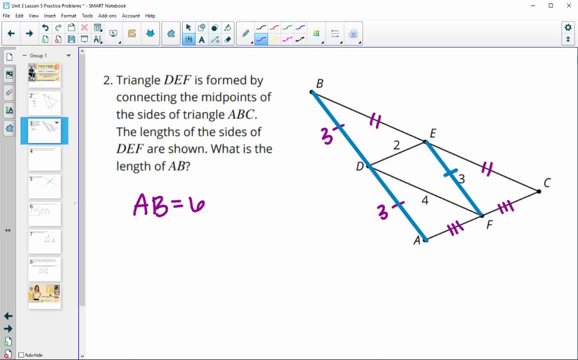 dilated by a factor of 2.. And we would also know- and this isn't part of this problem, but just a similar thing, so this is DE here. we would double that to get AC. so this one is 2,, so this longer one is 4, and then also DF: here is 4, so BC would be 8,. 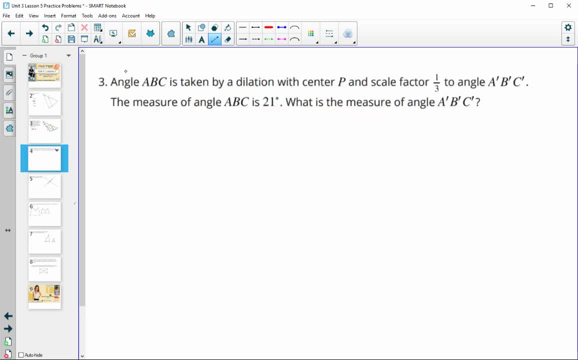 so those kind of go together like that. Number 3, angle ABC is taken by a dilation with center P scale factor 1, 3rd, 2.. Angle A', B', C' the original angle measure is 21 degrees. so what is the measure of the dilated? 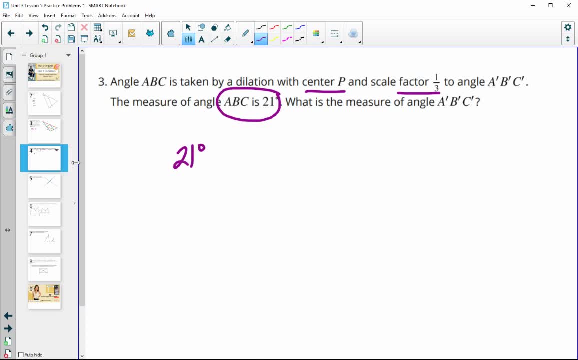 angle. We know that angle measures don't change in dilations, so the new one is still 21 degrees. Number 4, draw any two lines that could be images of line M by a dilation label, those lines N and P. So remember when lines are dilated. 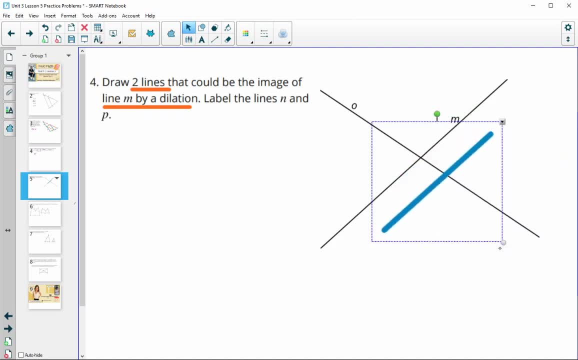 they're dilated to themselves or to parallel lines, so any of these lines would work, okay. So anything that you're seeing here, so you can just draw any two lines. they just need to be parallel to the original line M. so this could be one, this could be one, and then you just need to. 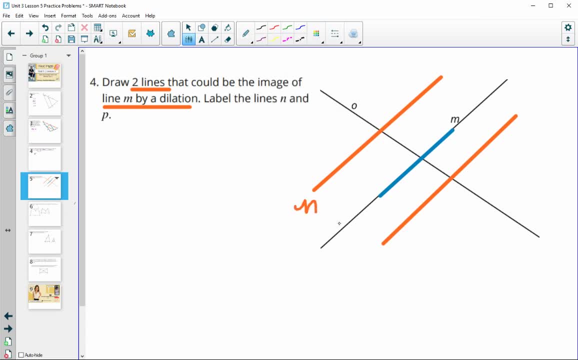 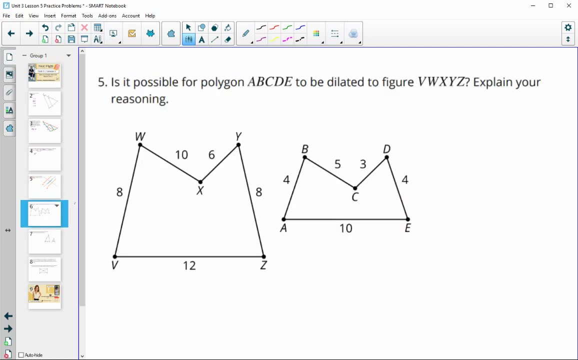 label those. And so it said: label it, one of them N and one of them P. Number 5 says: is it possible for these two polygons to be dilations of each other? So was this dilated And explain your reasoning? So kind of, look at the similar pieces and just check if they are being. 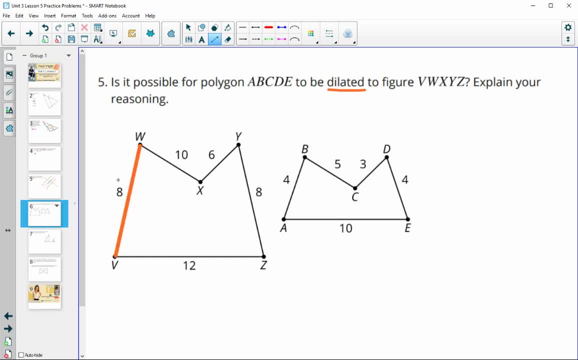 dilated at the same scale. So if we look at this one, this one's 8, and its dilated piece is 4, so we see a connection there of dividing by 2 or a scale factor of 1 half. So if I take 8 and I multiply, 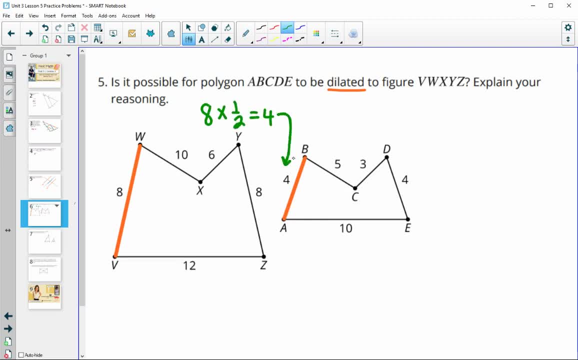 it by 1 half, I would get 4.. And so then that needs to happen with all the other pieces in order for this to be a dilation. So we can see: 10 goes to 5,, 6 goes to 3,, 8 goes to 4, those are all. 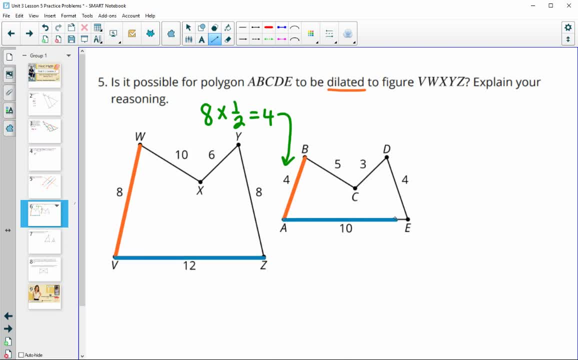 good, But when we take a look at this bottom one, VZ to AE 12 times 1 half is not equal to that 10, so then this would not be a scale, Or sorry, it would not be a dilation, because all the sides were not changing at the same scale. 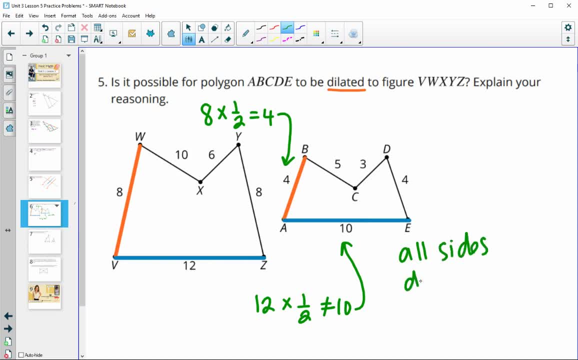 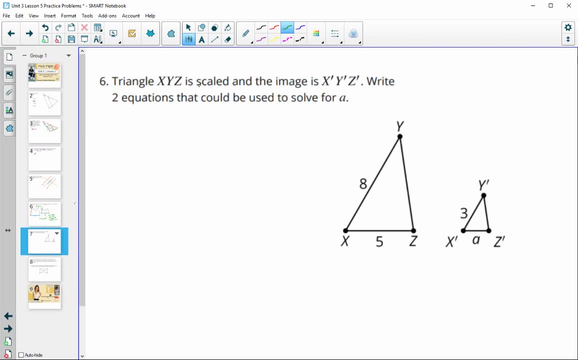 factor Number 6, triangle XYZ is the scaled image, or, sorry, is scaled and the image is X prime, Y prime, Z prime right. Two equations That could be used, So we know that these are similar and we just need to write two equations. 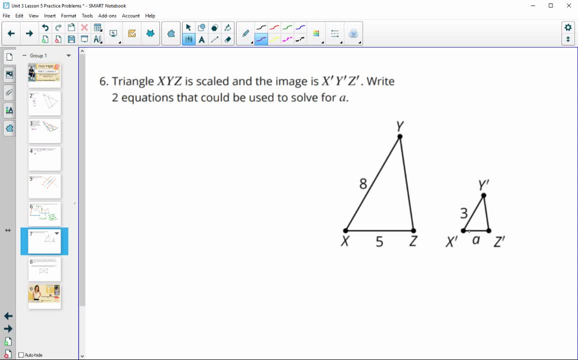 to solve for A. So one could be to compare A to 3. So I could do A divided by 3. And when I do that then I would just do a similar thing in the other triangle. So I went A divided by 3.. So now over here I'm going to do the similar pattern and do 5 divided by 8.. 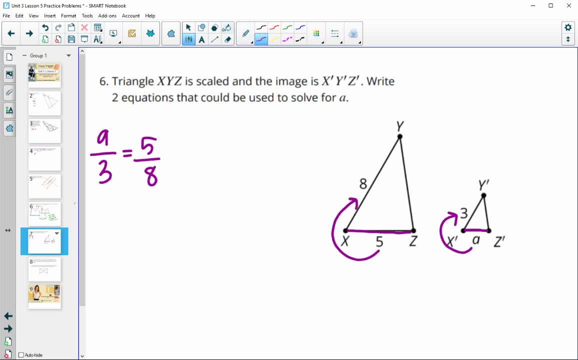 So there's one equation we could use. I could also just compare similar sides in the figures. So I could start by comparing A to 5. So I would do A divided by 5, and then I would compare, go back, So I started in the image. 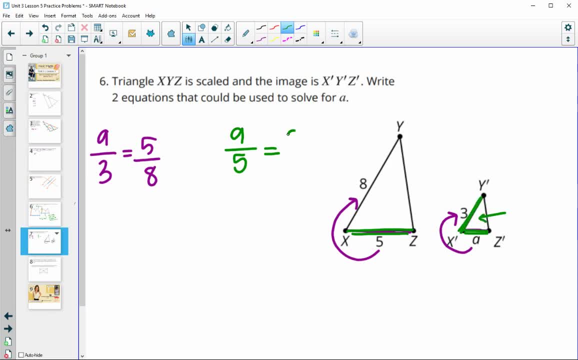 So I started here, so I need to go back to there. So then I'm going to go with 3 and compare that to 8. And then you could cross, multiply either of those to solve. And there's a bunch of other ones. 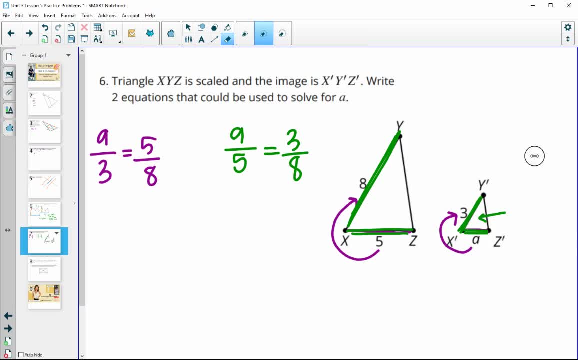 You could write- So this is not the only ones. So you could do like 8 over 3.. So I went 8 over 3.. So now I'm going to go 5 over A. You could have gone 8 to 5.. So 8 compared to 5, and then 3 to A. 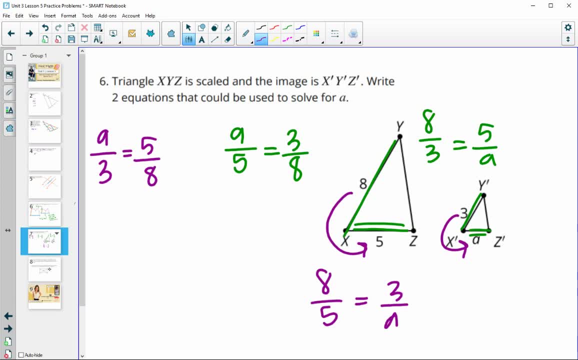 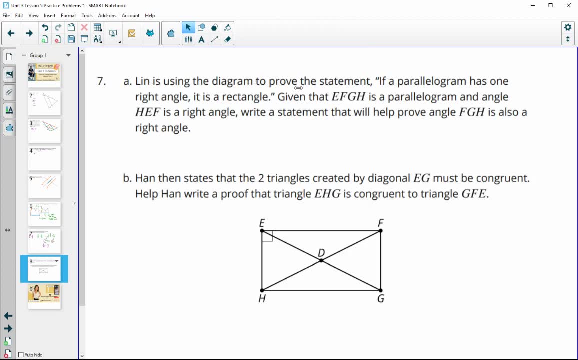 So there are a lot of other equations. That's just a few examples. In number 7, it says that Lynn is using the diagram below to prove the statement that if a parallelogram has one right angle then it's a rectangle. So given that EFGH is a parallelogram and angle HEF, that's pictured here. 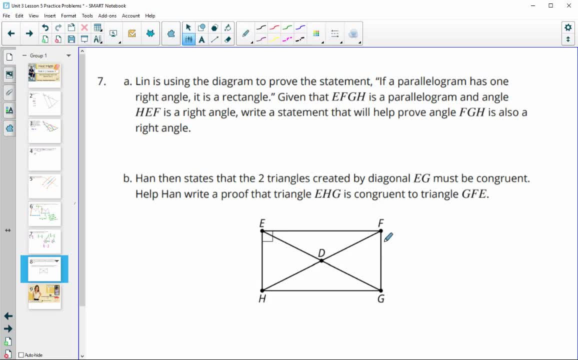 is a right angle. write a statement that would help us to prove that FGH is also a right angle. So how could we prove that this is a right angle? And that would be that we know That opposite angles in a parallelogram are congruent. So we know that. 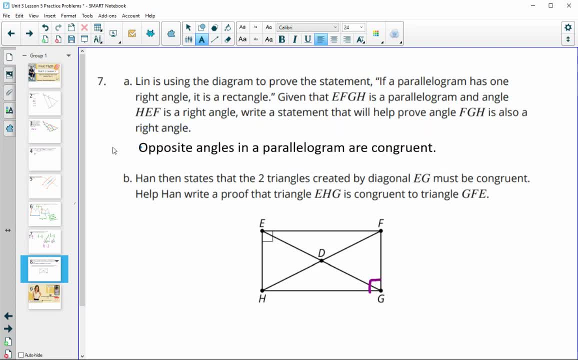 So if this one's the right angle, then we would use the fact that we know that opposite angles are congruent in order to prove that the other one is a right angle. Then it says that Han states that the two triangles created by diagonal EG are: 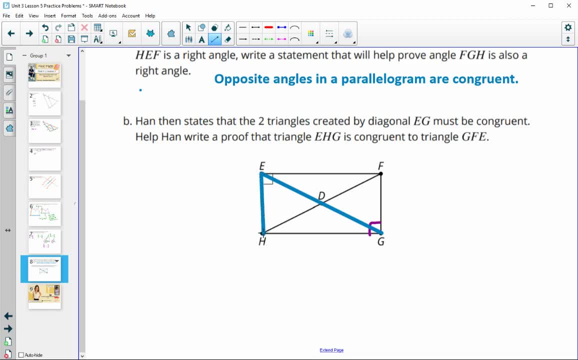 congruent. so let's help him write a proof. So we're trying to prove that kind of this triangle down here is congruent to this triangle up here, And how would we do that? So a couple things just as we start looking into this, So things that we know — before we start writing it. 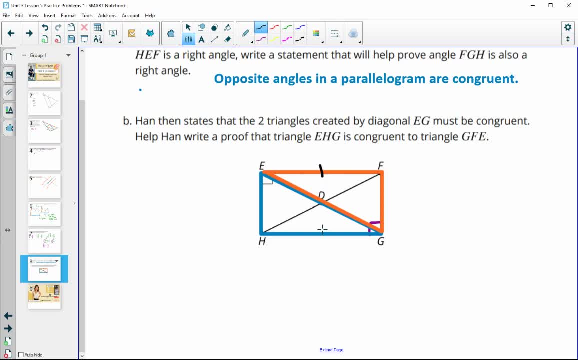 out things that we know. we do know that opposite sides in a parallelogram are congruent. So we would know kind of these top, top and bottom are congruent and left and right are congruent. And then we also know that EG is in both the orange and the blue triangles. 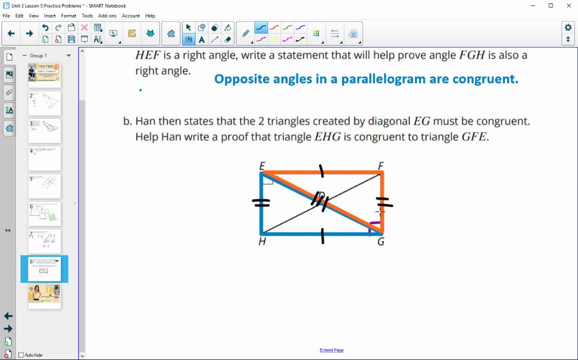 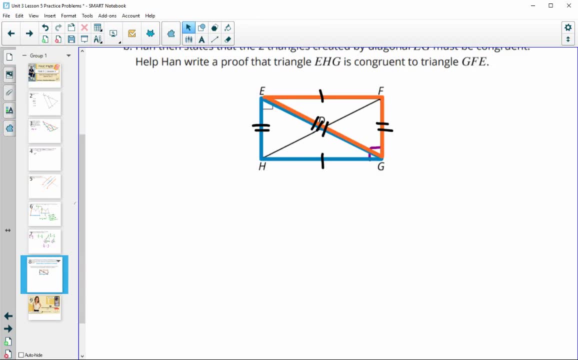 So that's going to be congruent to itself, And then that would help us prove the triangles are congruent, because we know all three sets of sides are congruent. So that's kind of our plan. So now we just have to get that written out. 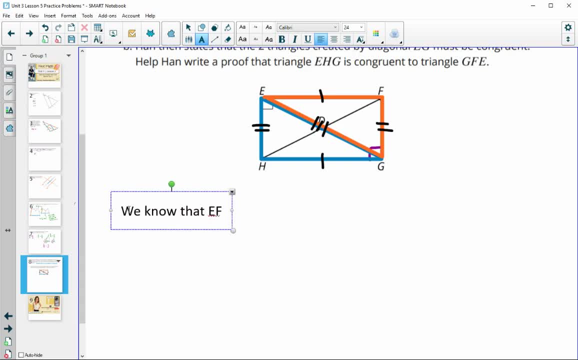 So we know that EF is congruent to HG and EH is congruent to FG because opposite sides of parallelograms are congruent. So that was that, top and bottom, left and right. We also know that EG is congruent to EG because it is the same segment. 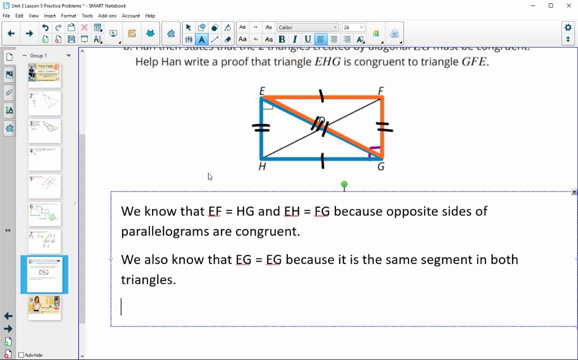 Both triangles And then therefore Triangle EHG is congruent to triangle GFE by side side side. Triangle congruence: Triangle HG is congruent to triangle GFE by side side side. 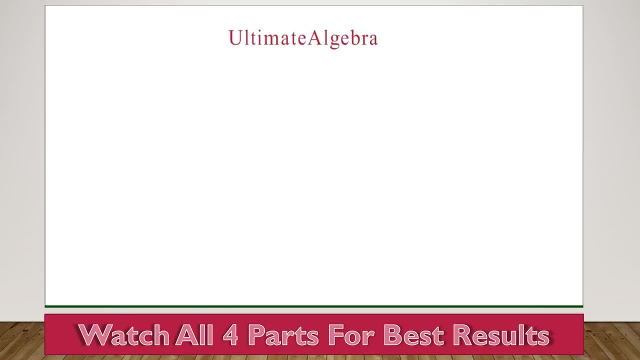 Welcome to another video from UltimateAlgebracom. In this video, we will be introducing ourselves to word problems. Specifically, we will familiarize ourselves with the implication of different words and expressions. Being able to translate the various expressions to math forms 90% of the requirement to be good in solving word problems. 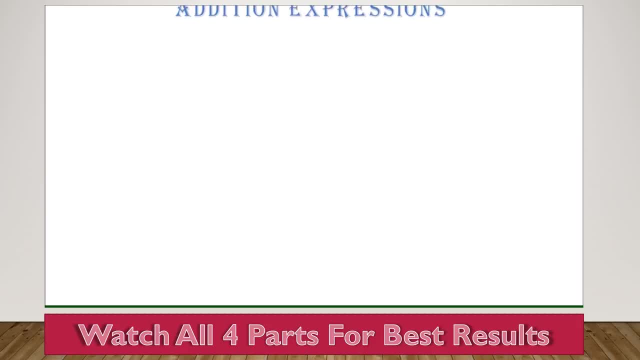 Let's look at the most common expression used: addition expression. The following expression implies addition: 1. Increased by 2, more than 3, added to 4,, some 5. Comparative words that denote more than Longer, faster, taller and so on. 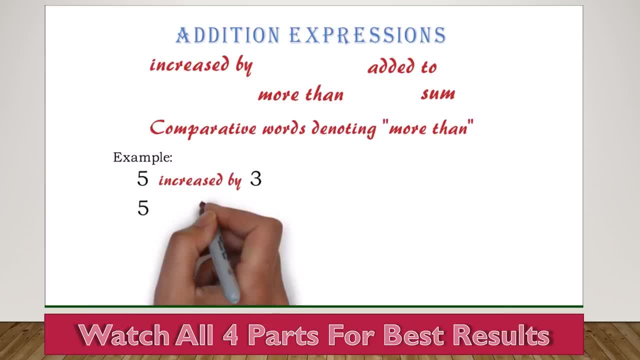 If we have 5 increased by 3,, this is the same as 5 plus 3.. If we have 2 more than 8, this is the same as 8 plus 2 or 2 plus 8.. You can interchange numbers in addition. 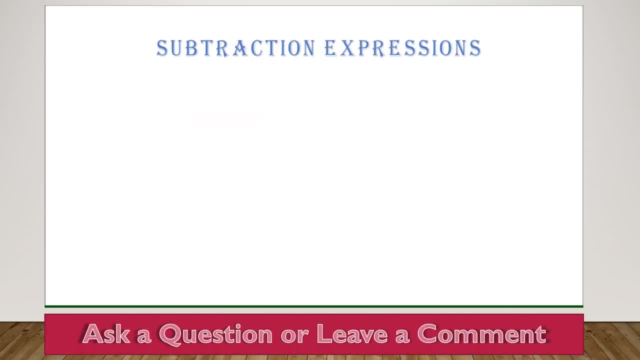 Subtraction expressions. The following expressions implies subtraction: 1. Decreased by 2, less than 3, taken from 4, subtracted from 5, difference 6. Comparative words that denote less than Smaller, shorter, slower and so on.